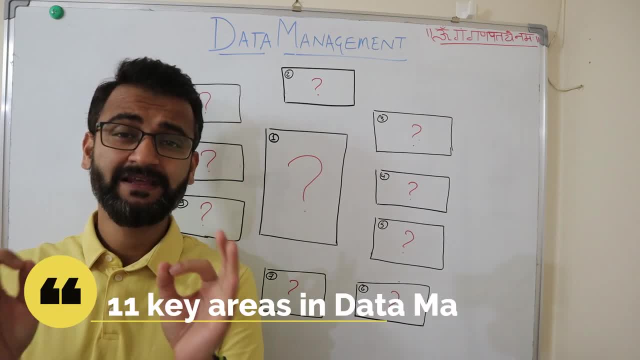 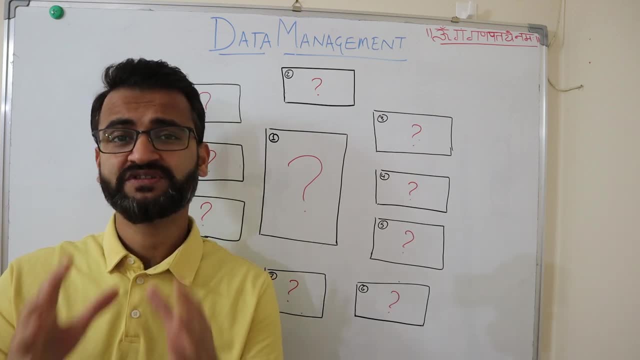 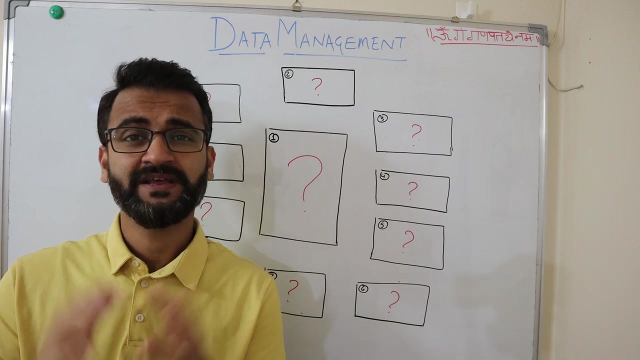 But if we go by the standards, there are 11 clear and precise areas which have been defined And these 11 areas actually make sure that the whole data within the industry, within your company, you know, is working, is managed properly, is secure, is reliable and is effective. 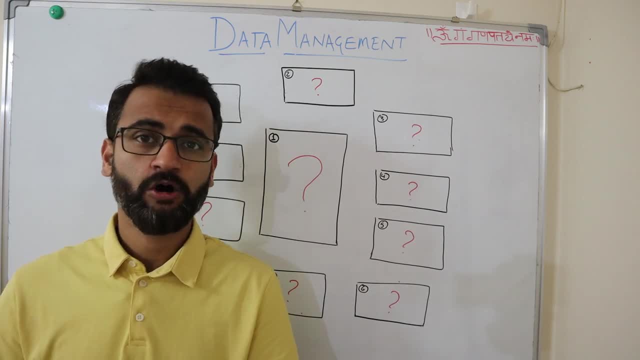 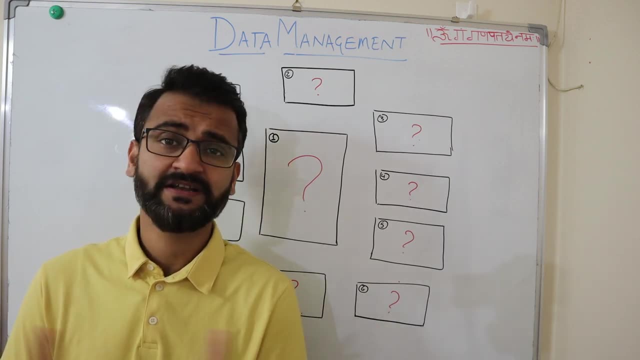 So when you are starting your journey in the field of data, or if you are already working in the field of data in any role, be it data engineer, data scientist, data analyst- I'm pretty sure that you would be working in one of the fields of data management. So when you are starting your journey in the field of data, 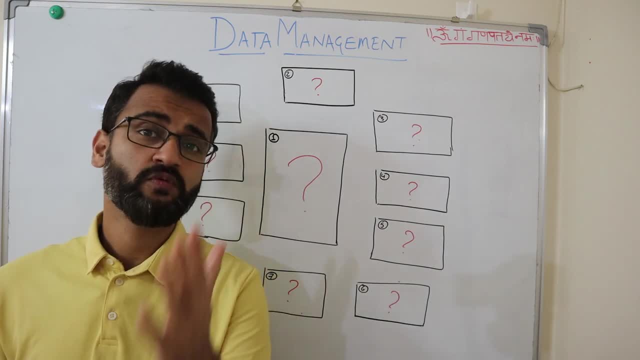 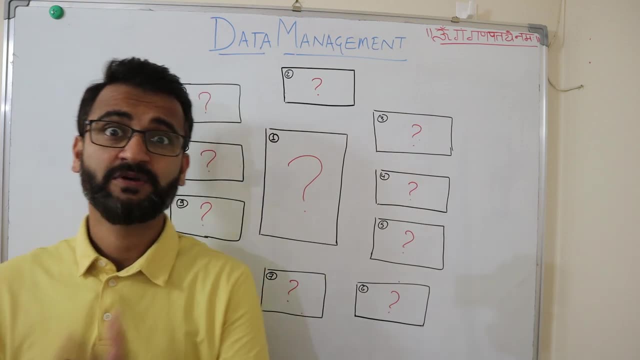 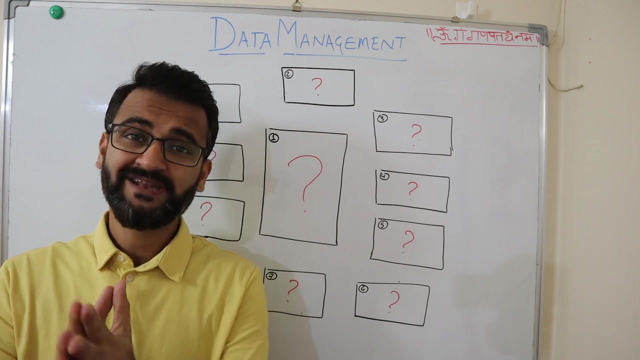 one or many of these areas. And, of course, if you want to start your career in the field of data, it is very important for you to learn about these 11 areas, because this would come to you from time to time within the specific role you are working in. So we'll start our video by understanding all these different concepts. 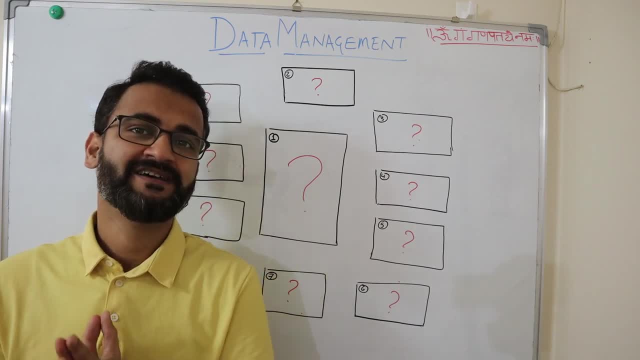 and specific features of every area in the field of data management. I'm sure this is going to be an interesting video, So without further ado, let's get started. Thank you, friends. If you're new to ITK Funded channel, we make IT interesting for everyone, be it IT or non-IT. 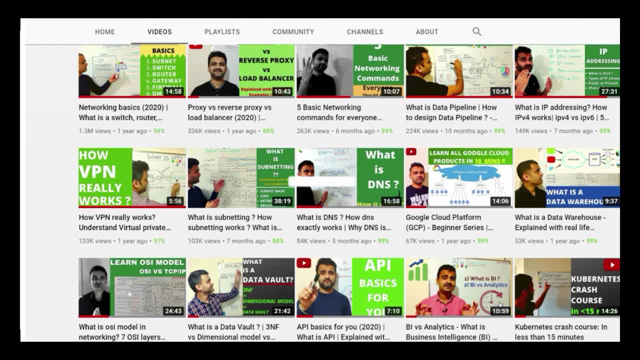 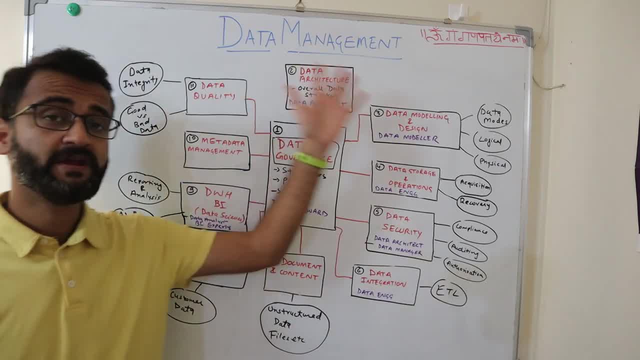 We discuss all the latest tools and technologies, products, productivity hacks and career tips on this channel. So if you are new and if you like the content, do consider subscribing. Thank you. So, friends, this is data management and the 11 data management areas. I have depicted it in this pattern. 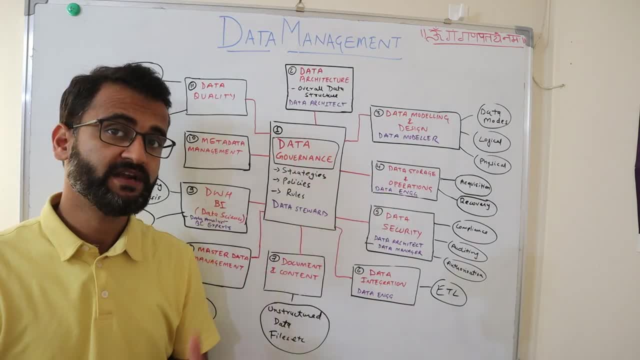 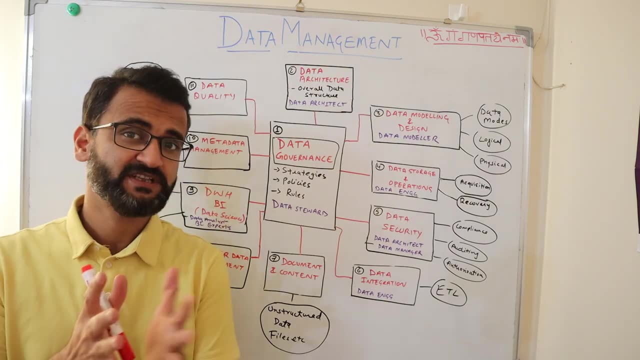 but we'll go through each and every area one by one and quickly understand what exactly That area does and also some key roles in the IT industry which belongs to that specific area, although a lot of roles are there and one rule can span across multiple areas. 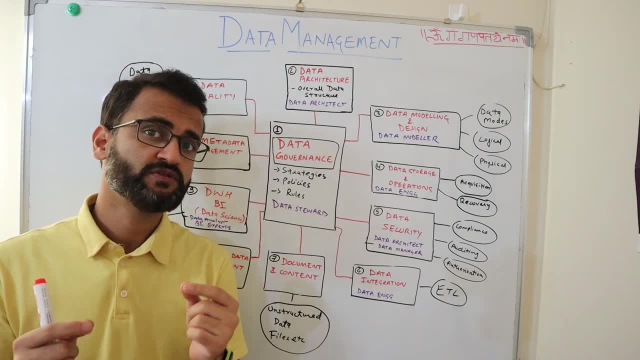 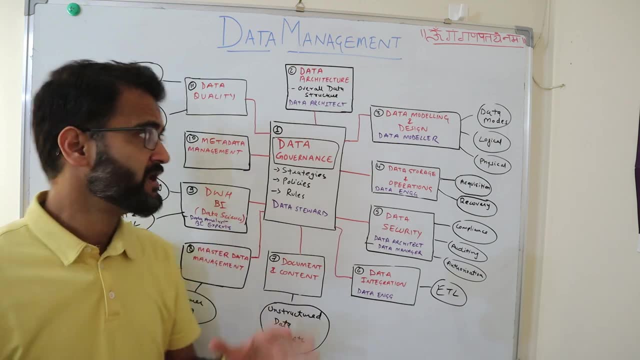 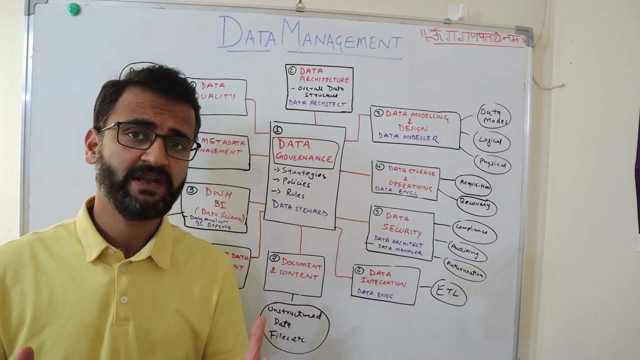 But then we will try to understand certain specific rules which fall into one specific area. So, to start with, at the center of any data management lies data governance. Now, data governance in itself is not something very technical as far as data management is concerned. 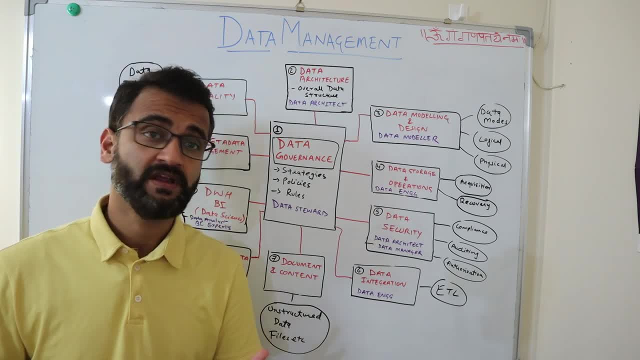 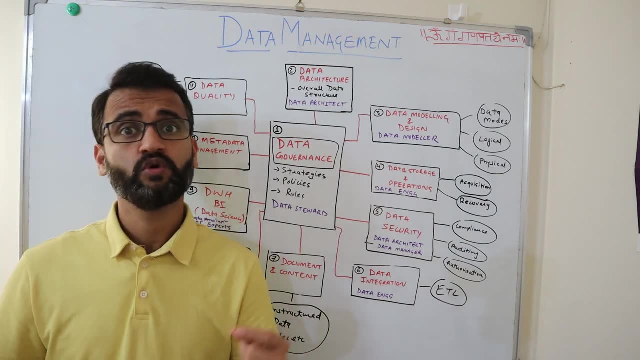 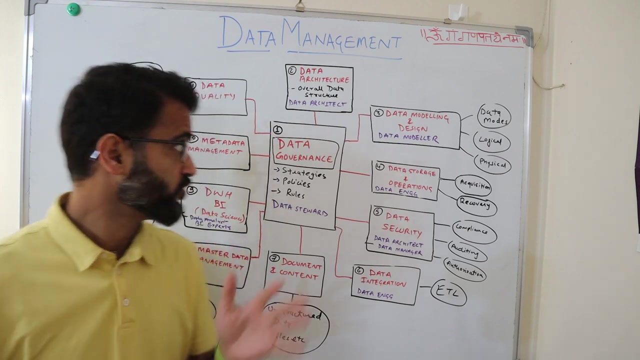 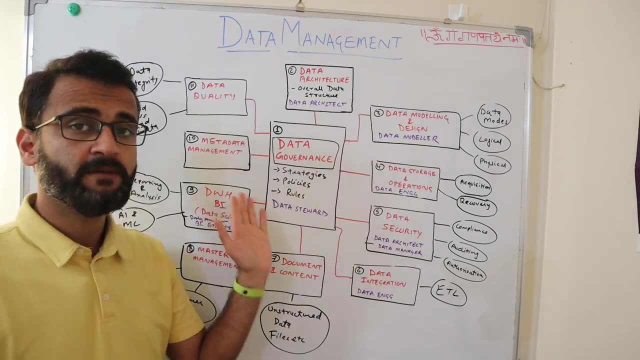 is concerned, but it does what a government does for a country. so it creates strategies, policies and rules and a framework. it defines a framework with which data would be, you know, managed and controlled and maintained within an enterprise, company or industry. so data governance sits, you know, at the center and it connects with every other aspect of data management to, in totality, all. 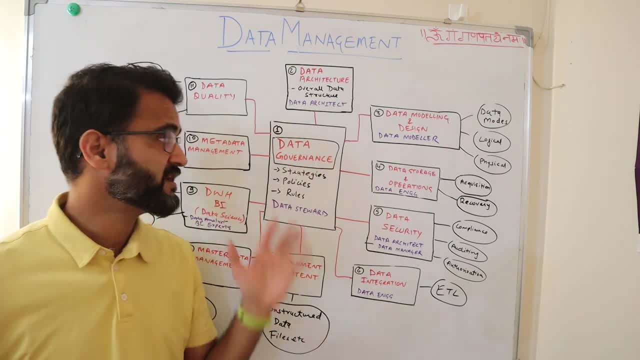 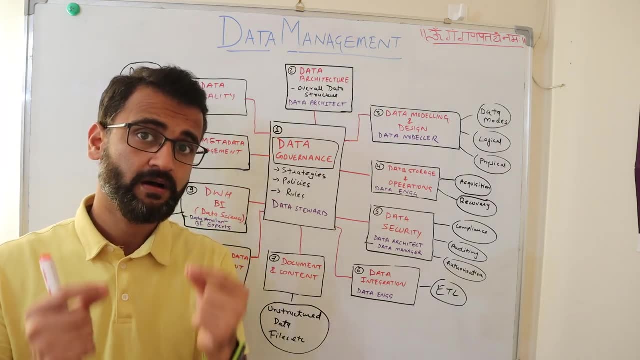 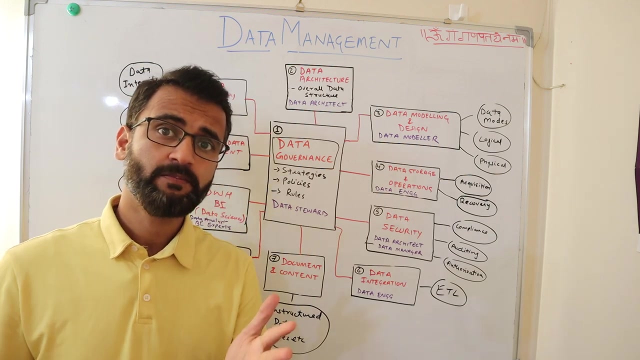 the other 10 areas connects in some way or the other with the data governance. so data governments sit at the middle, and one specific role which comes up when we talk about data governance is its data steward. so it's the responsibility of a data steward to five define the policies and the 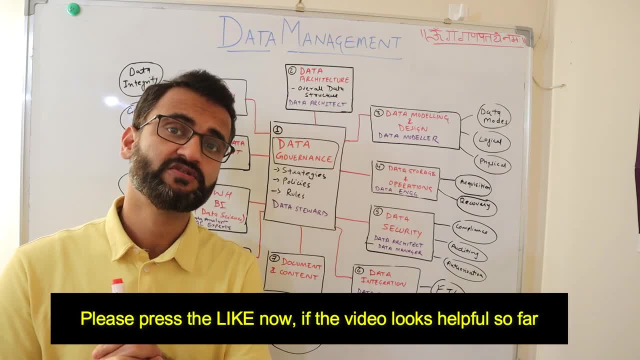 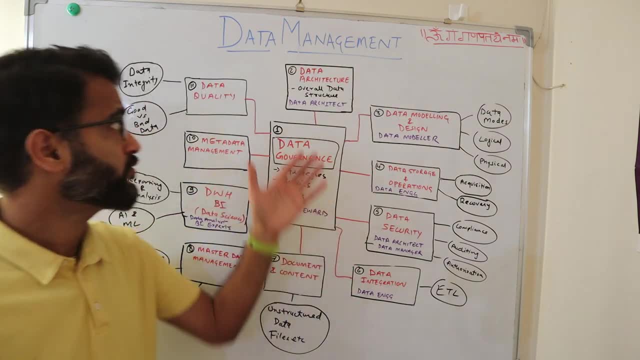 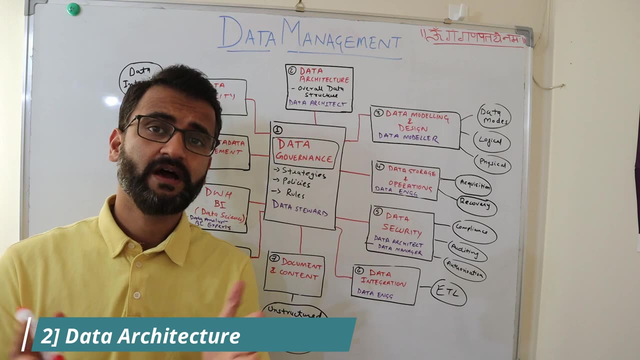 rules and regulations with which you know he can lead this whole data governance processes. so this is our number one area, right at the center. now to start, you know, in a clockwise direction, the very first thing which comes is data architecture. so what is data architecture? so in data architecture, there would be some chief data architects in your company. 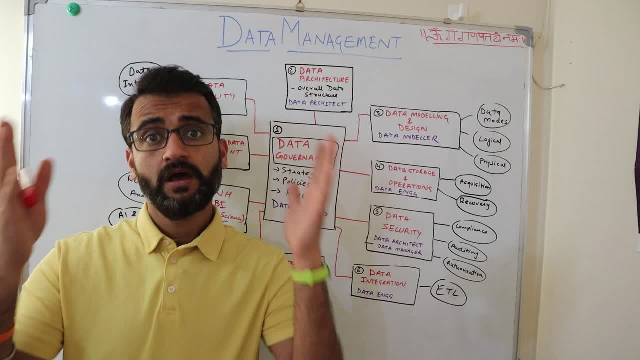 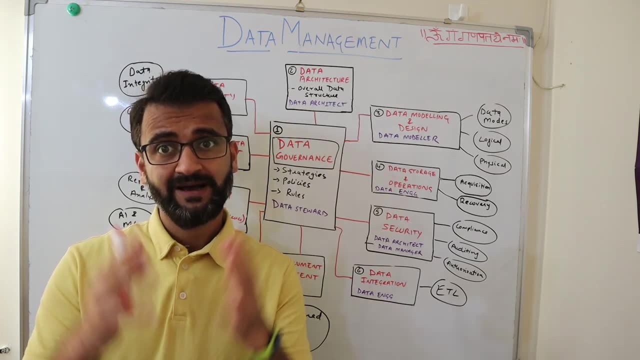 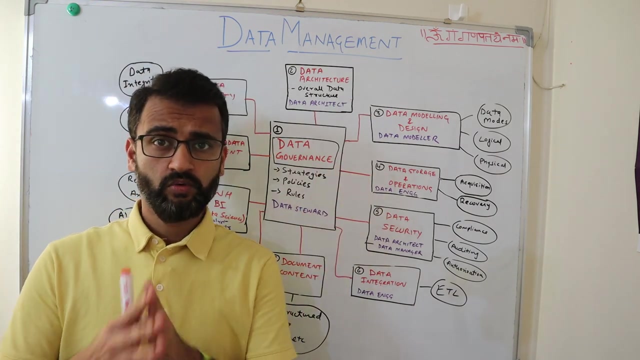 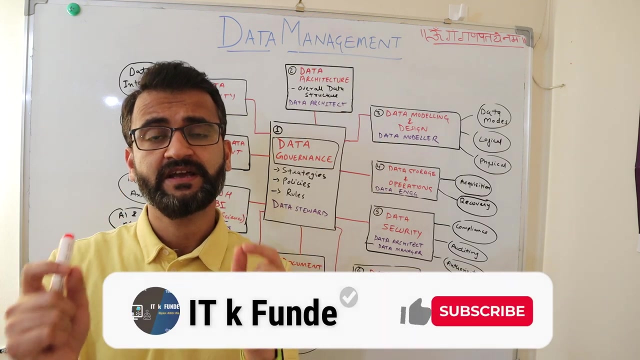 who would decide that, how the data for that particular company will fit into a specific design or architecture. so these are those people who define those kind of you know data architecture and designs, and that's why a data architect- or, in some companies, we have Chief data- who, and their responsibility is only to you know, manage and define what kind of data architecture. 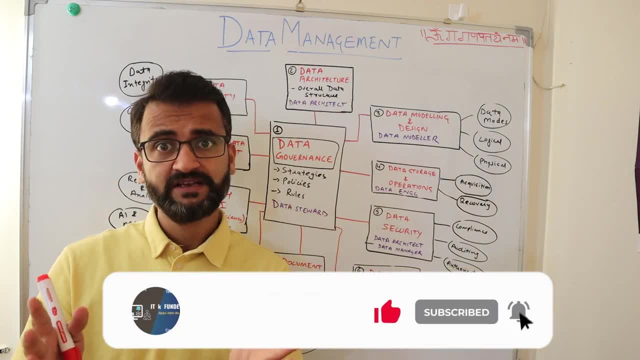 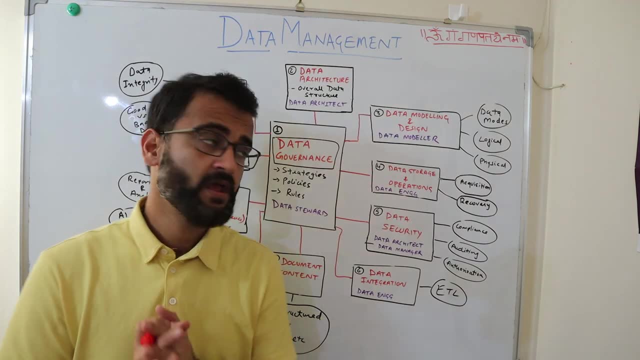 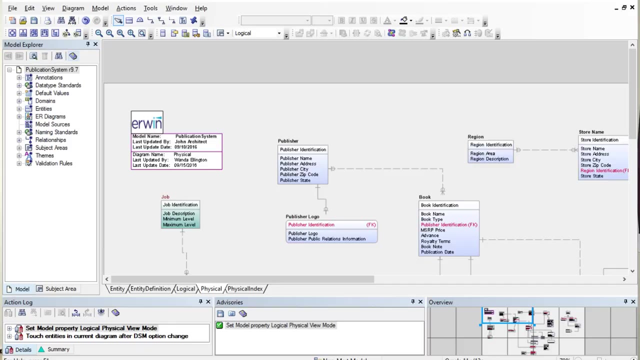 this particular company will follow and, based on that architecture, other disciplines follow that particular pattern and tries to define data in that particular shape. so data architecture is a very important field and there is a very good product, irwin data modeler, which is very old tool but very commonly used till today, and it is a license- licensed software wherein 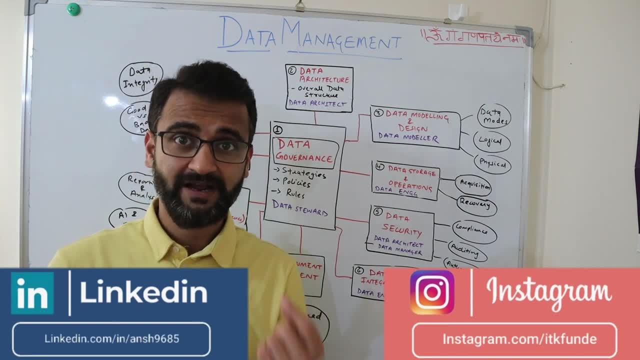 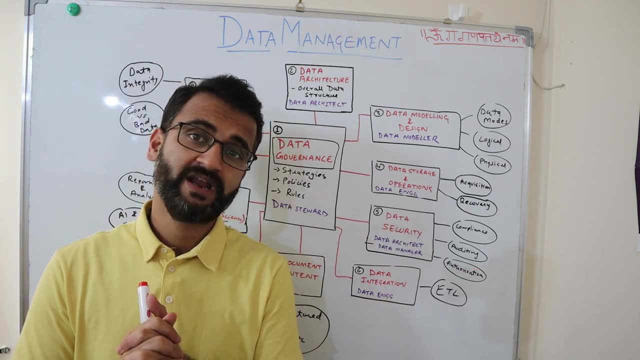 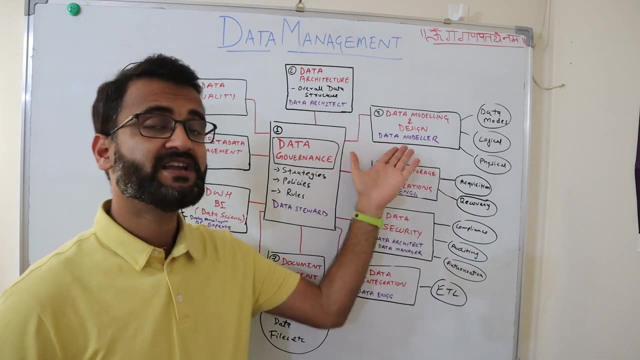 you know the there would be a license given to all the data architects and those data architects could then go into irwin data modeler and manage and, you know, do their activities as a data architect. so a very good tool. so a related branch to data architecture is data modeling and design. 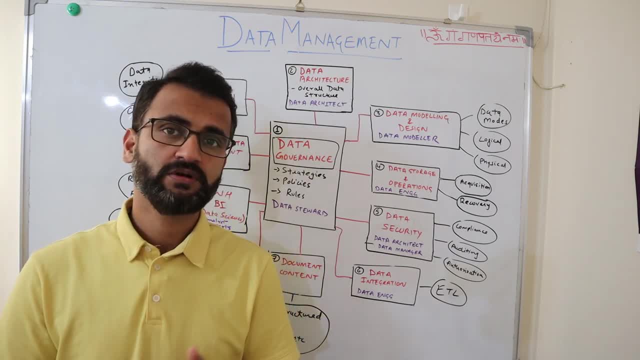 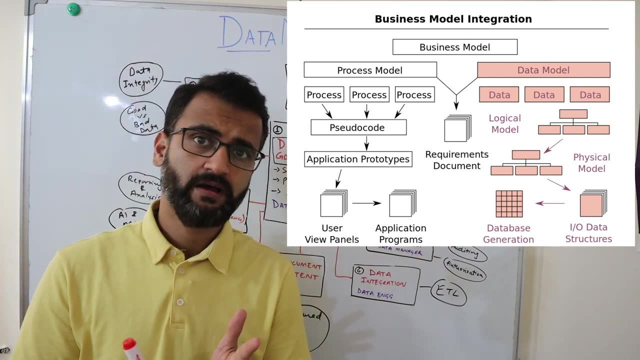 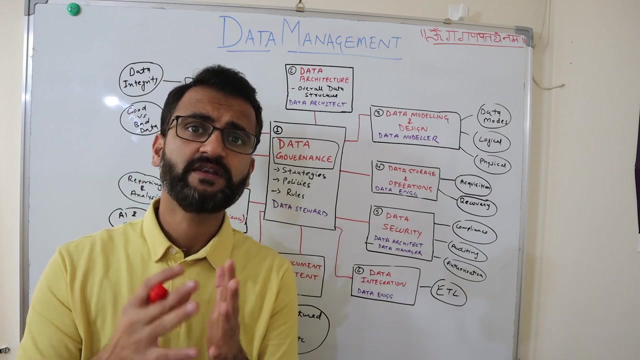 so within data modeling and design, the conceptual data model, the physical and the the logical data model is defined and based on that particular data model. all the data extraction, acquisition, storing, everything happens around that particular data model. So suppose there is a new project which has come up which has to develop something for 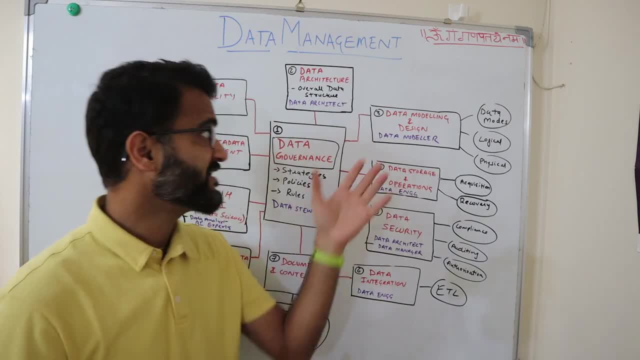 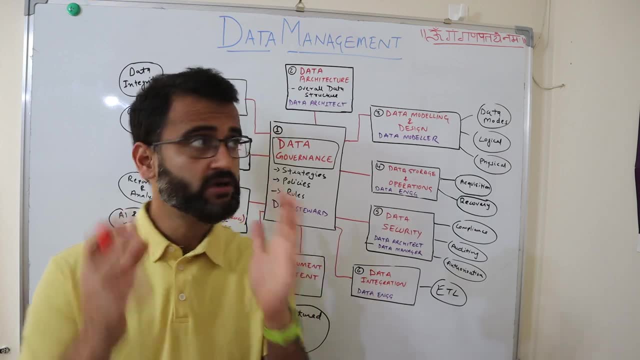 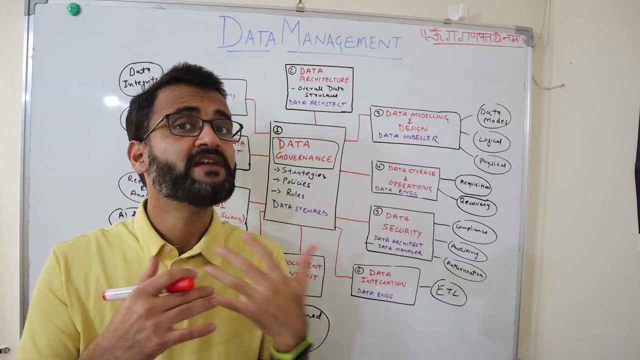 example, a report. so they need to consult the data modeler and understand what kind of a data model can be fit into this particular use case, and that data model should be in line with the data architecture strategy defined by the data architect. So you see, everything is very interrelated in this area. 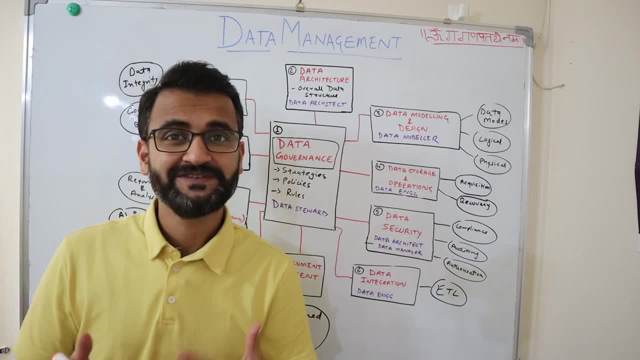 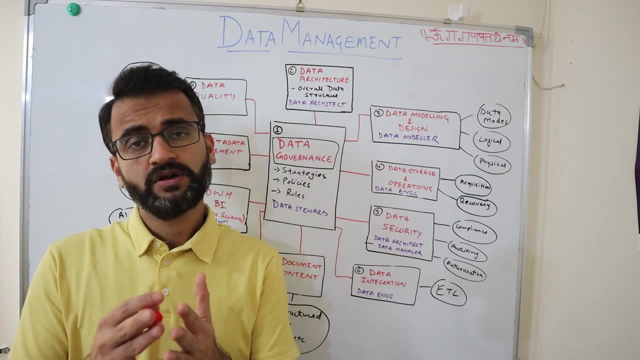 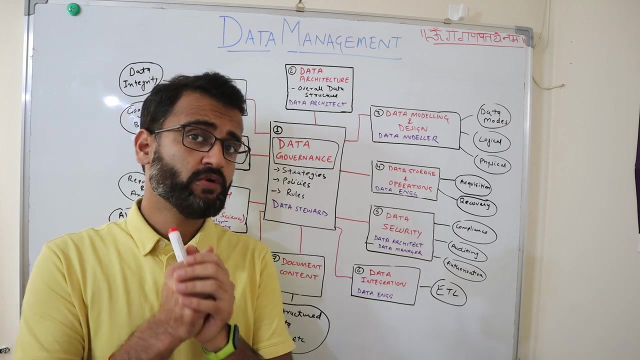 Coming to the fourth one, which is data storage and operation, which is very close to me. what I do very closely because, you know, in data operations you are the owner of how the data- you know data- is acquired, maintained, recovered and ensuring that your end-to-end 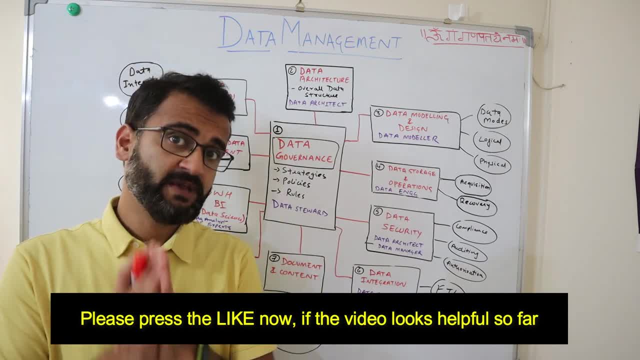 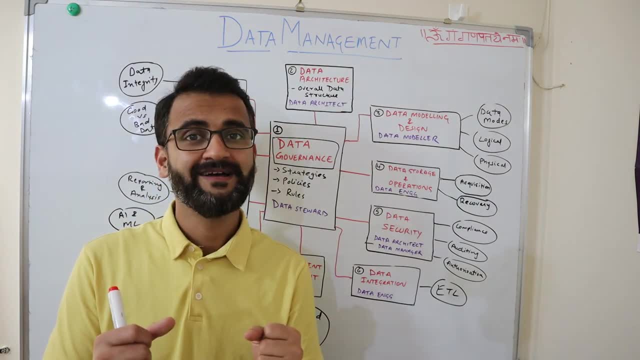 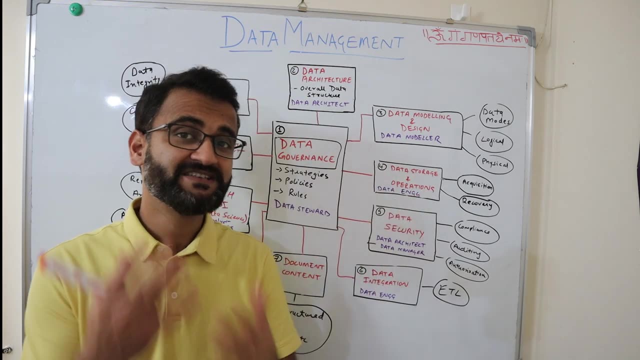 data pipelines are running on time And it is being maintained correctly. So data storage and operation is all about how you maintain and store your data in an enterprise, And one very important role which fits into this particular area is data engineers, because data engineers are the ones who are very much responsible for these kind of activities. 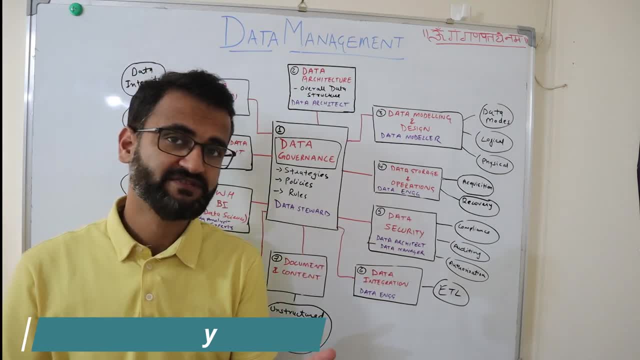 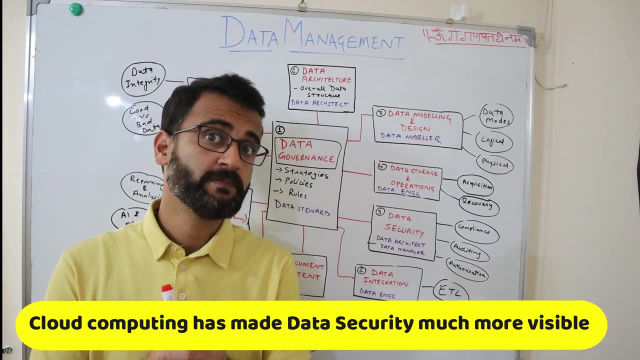 So, coming to our fifth area, which is data security. the name is self-explanatory. It talks about all the compliances, audits and what kind of security mechanism Which needs to be placed, all kinds of data authorizations which needs to be done. 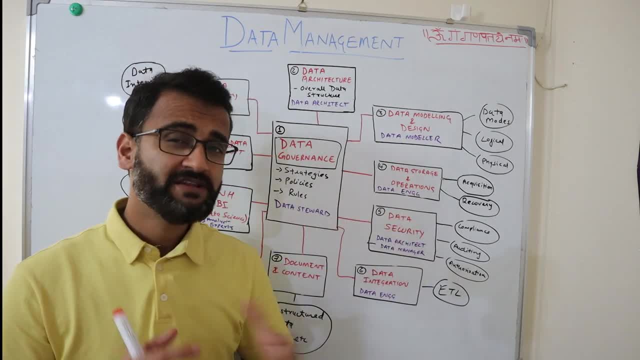 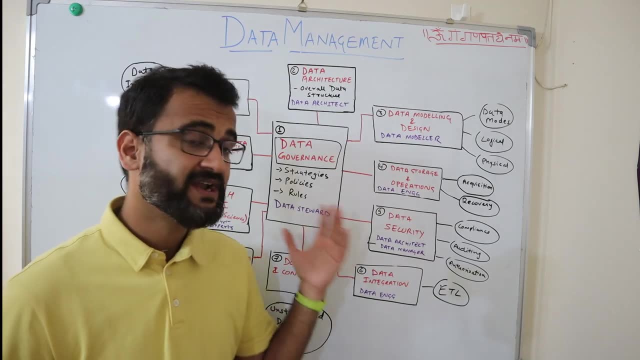 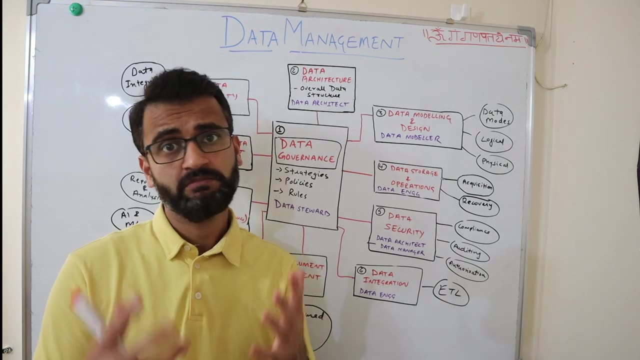 Everything related to that belong to data security. Now, there is no specific role which I have heard of which is very specific to data security, but what generally happens is that your data architect, your data manager or, for example, your data engineers, you know they lies with your respective security team. 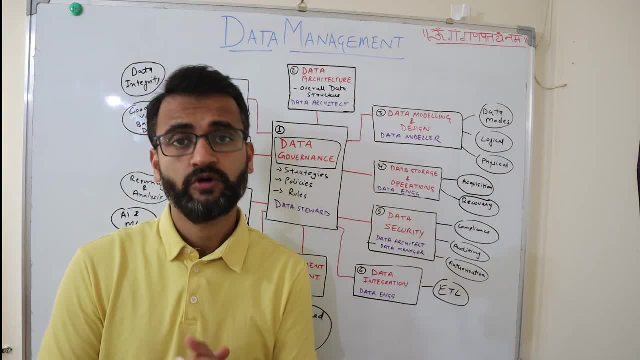 And then there is a data security framework which is defined for the overall security. So, by the end, this is all about how we can manage our data. How do we manage our data? How do we manage our data? This is a concept for this program. 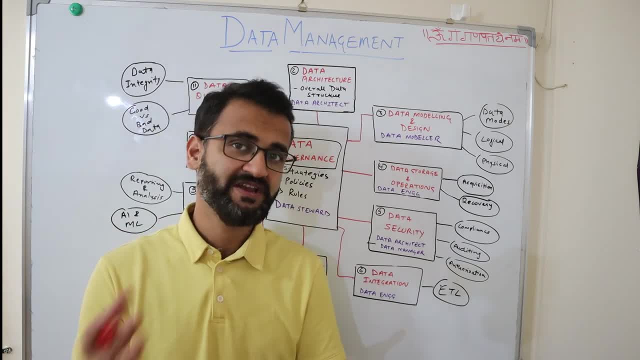 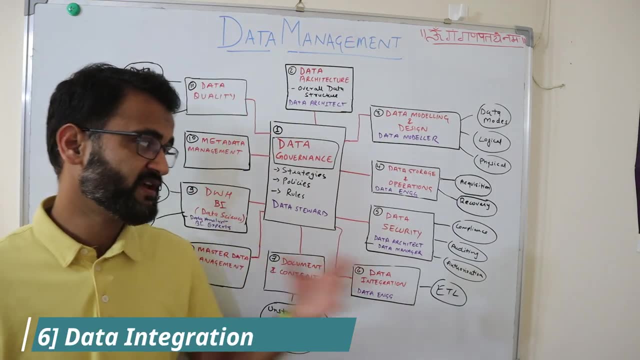 You know, you look like you know I'm at the top of your mind. Okay, let's go to the next question: company. but yes, it varies from case to case, so I'm just sharing my experience on this. so, sixth one is data integration. again, here, there is only one word, which 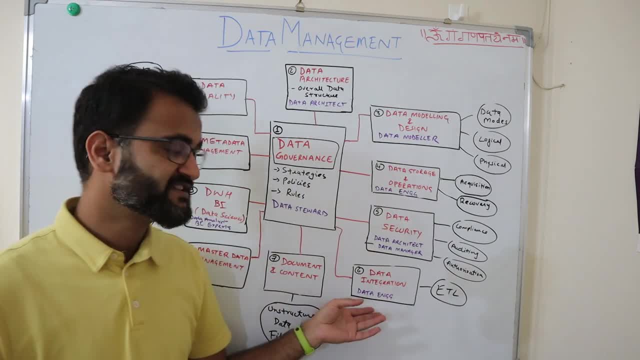 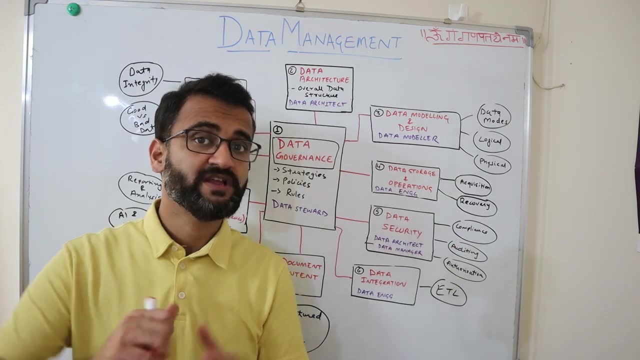 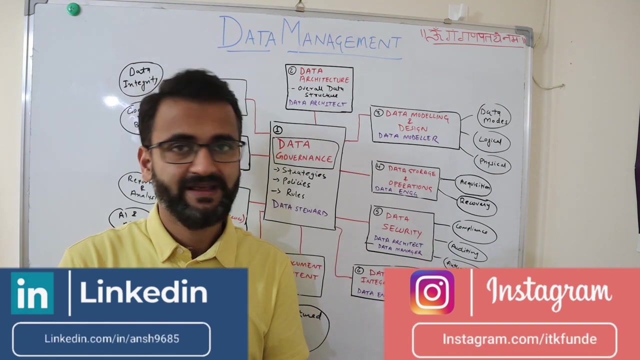 will explain it very simply- is ETL. so data integration is all about creating those integration pipelines so that you know how the data will be acquired from the source and then how it will be loaded in the destination. so this whole integration layer has been set up. so, yes, that is pretty much what happens within. 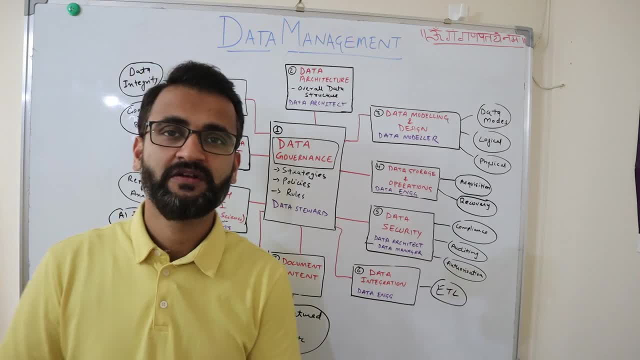 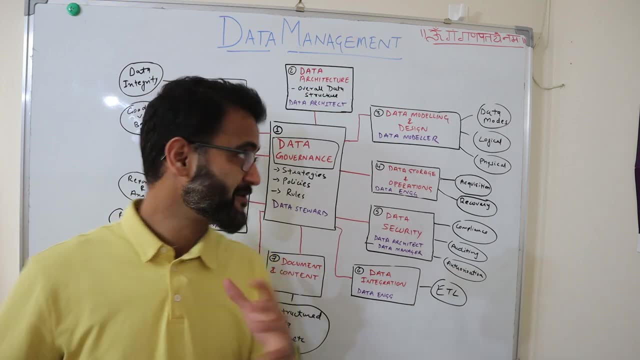 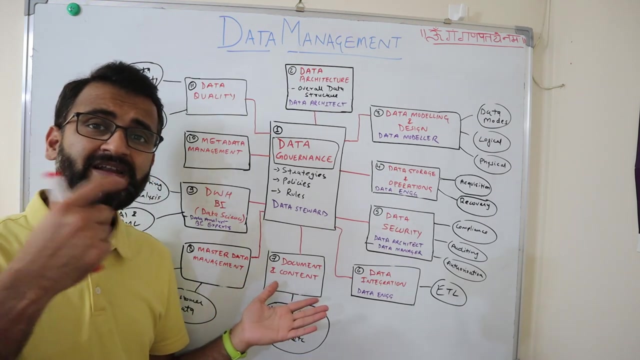 data integration. again, data engineer is a very prominent role and that's why you you see, data engineering is becoming so important, because data engineer is a person who covers a lot of these areas. document and content management is again a very important area and it relates to managing all the unstructured kind of 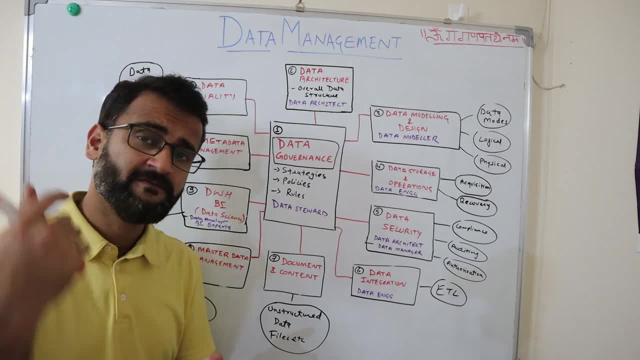 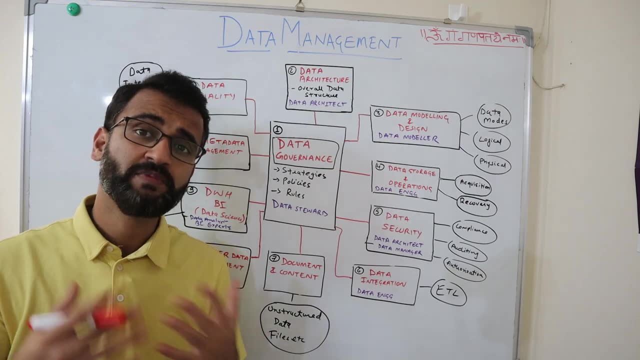 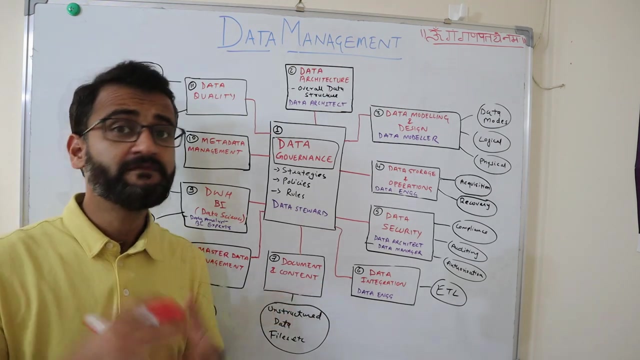 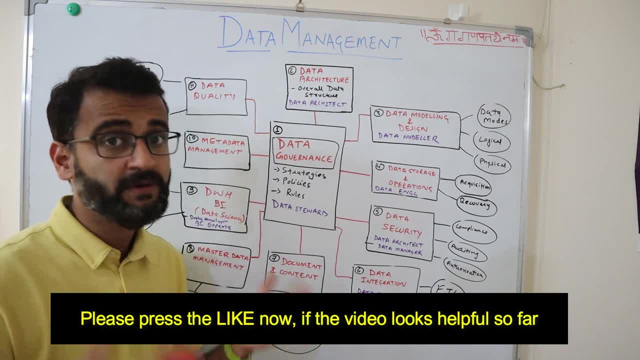 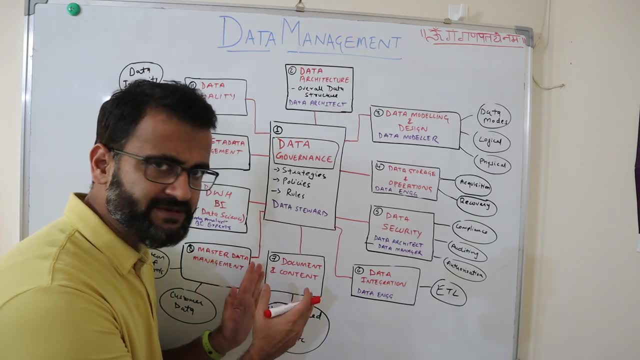 a relational kind of a data, but, yes, all the unstructured data, but still a crucial information, is managed under this particular area, not a very prominent area, I must say. there is no specific role which I can, you know, relate to this, but then it generally falls into. 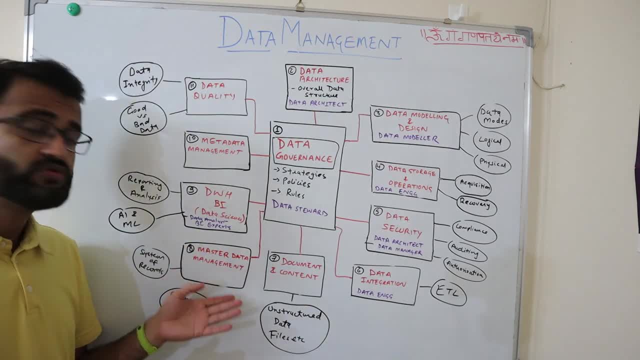 you know specific role which I can you know relate to this, but then it generally falls into the bigger picture. so, coming to the eighth one, which is master data, the bigger picture. so coming to the eighth one, which is master data management, it is a very important area in terms of this overall data. 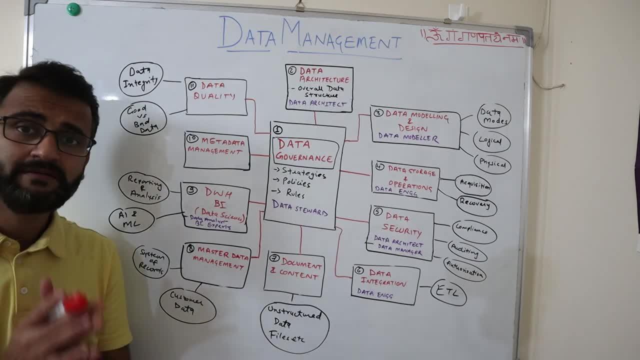 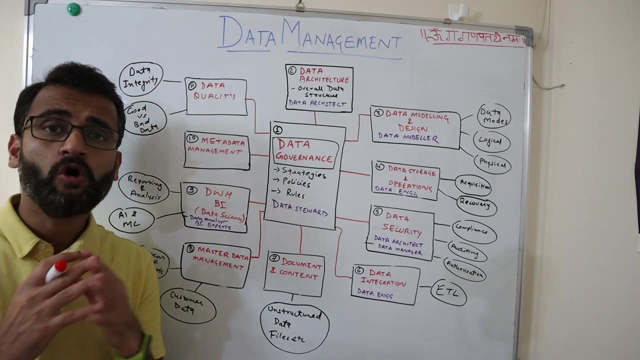 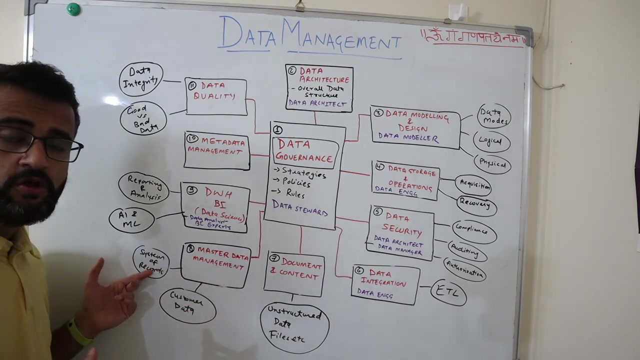 management framework, because your master data management ensures that you are managing and maintaining the quality of your master data. now, what is a master data? master data is, you can say, kind of dimensions or kind of entities, which defines all, all of your business processes, processes. so take, for example, your system of records, how the data is coming. 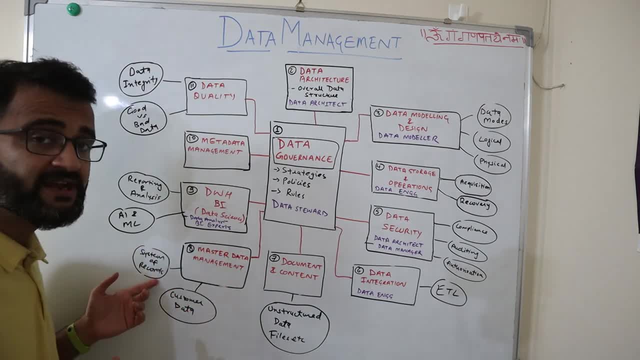 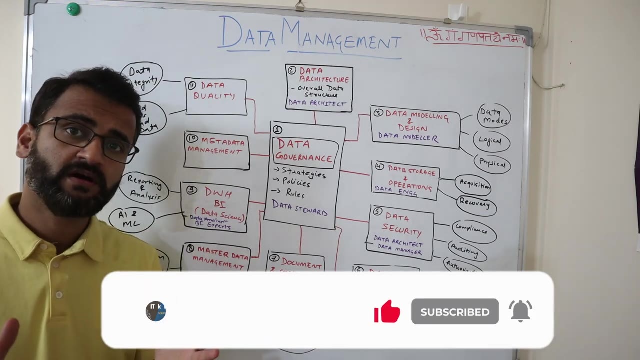 into the system and with what all entities this particular data is getting into the system and with what all entities this particular data is getting connected. that's what master data management is all about. one very good example to explain master data management is your customer data. so suppose for Amazon customer is a very important. you know dimension and 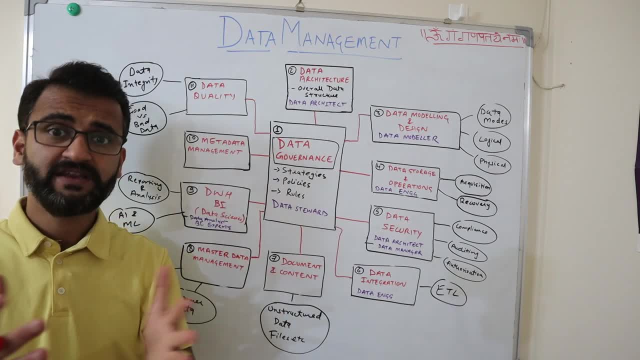 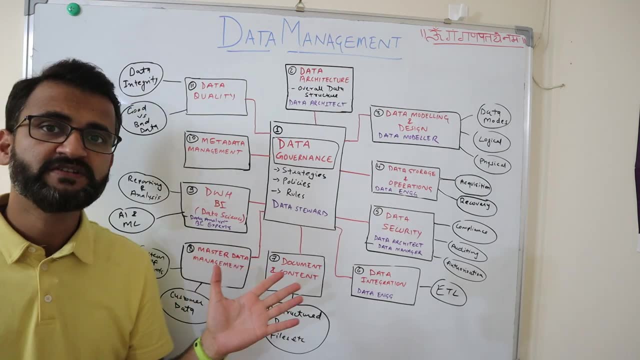 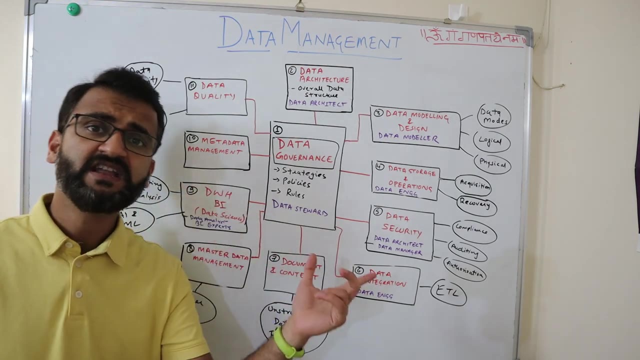 maintaining customer data uniquely and very, very clearly across the enterprise enterprise is very important because, suppose, if the customer data is managed by two different business teams and they are not interrelated, there is no master data to say that this is the same customer which has recently bought something from Amazon and the marketing team. 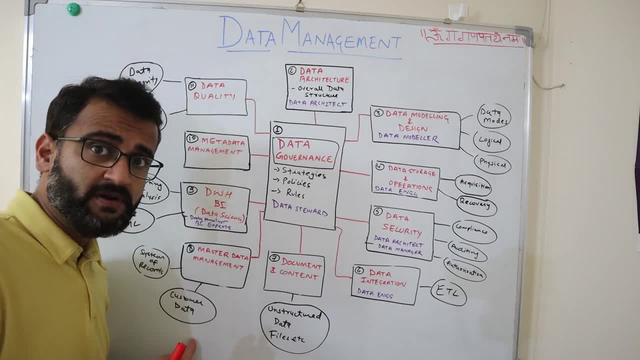 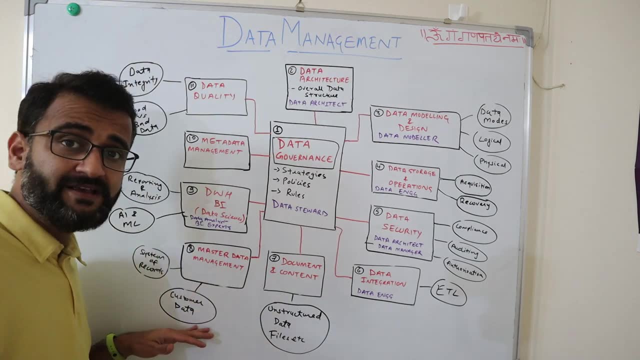 is again sending the campaigns to that particular customer without knowing that that customer has already bought that product, then that's a waste of time and resources, right? So in that case, if you have a common master data where you are managing all your customer, 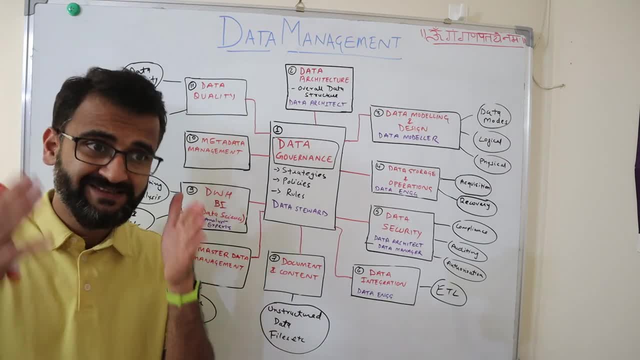 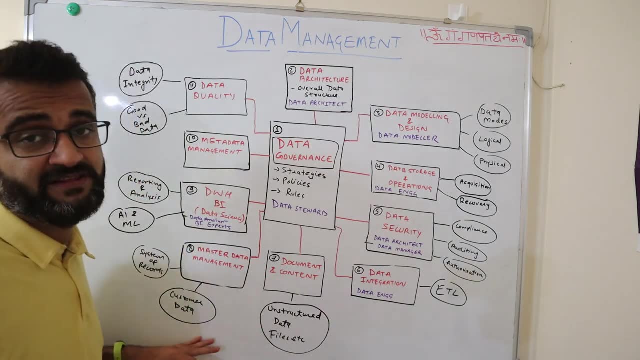 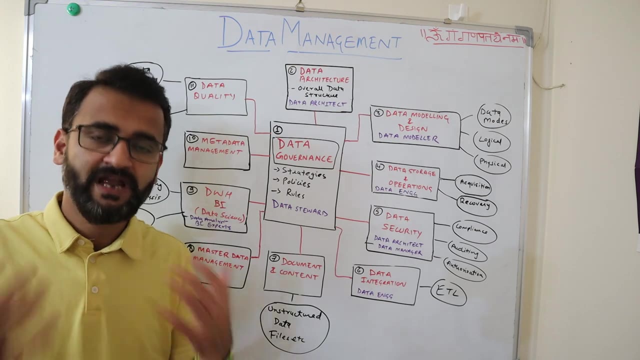 records, then it will help you identify that this customer has been targeted and then there is no point of going again for the same product for the same campaign with the customer. Just an example. It's a very big area, So let me know in the comment section if you need a specific video on master data management. 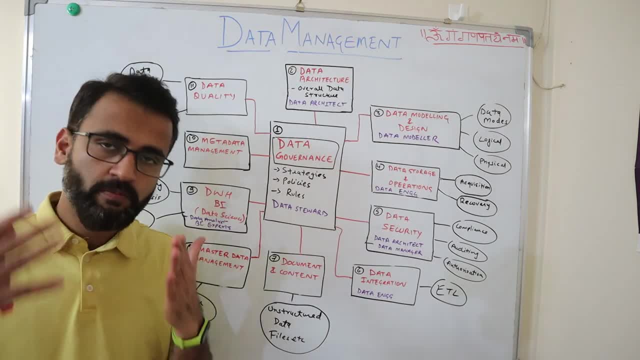 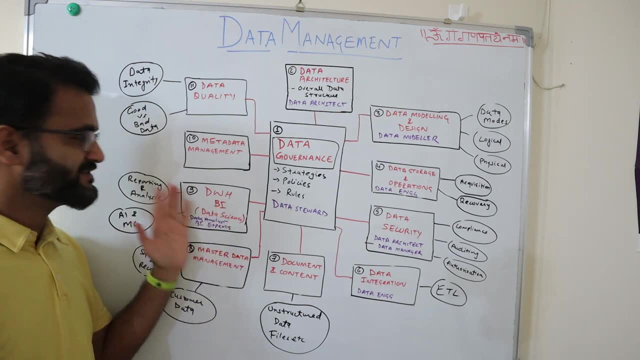 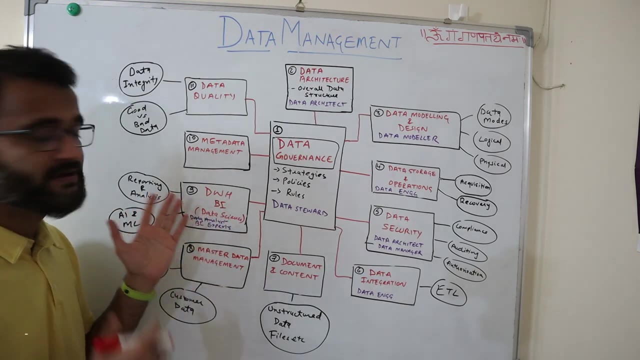 I'll do my studies and I'll try to make some elaborate video, specifically on master data management. Now, coming to my bread and butter, because this has been my core in area ever since I entered IT industry, which is data warehousing and business intelligence. 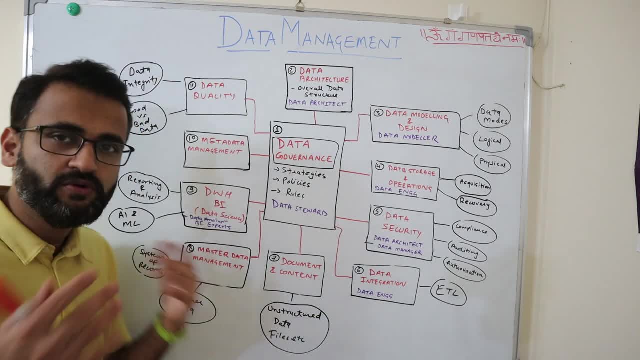 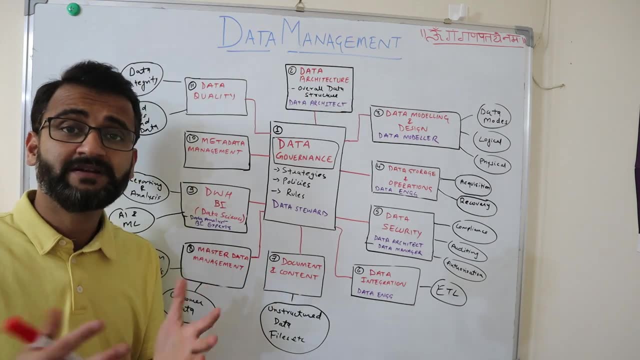 And I have made several videos on this, So I won't spend too much time on this. But again, everything related to your reporting, your analysis, anything related to storing the data in a centralized data warehouse, everything related to that becomes a part. 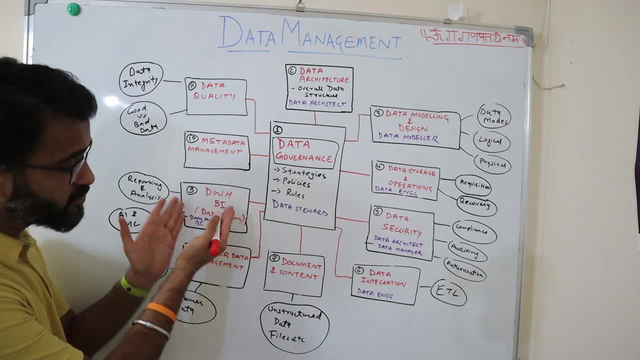 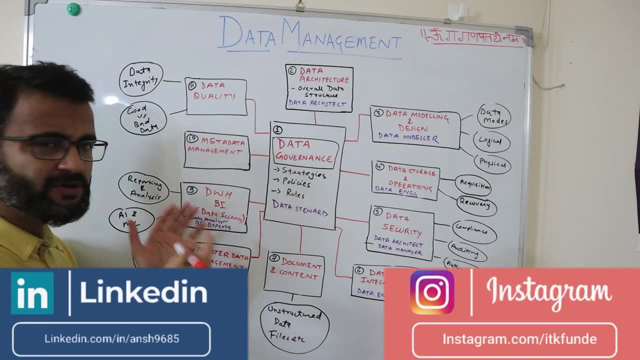 of your data warehouse and business intelligence, But I have now also added data warehousing and business intelligence, data science, into it. I have not kept it as a separate area, although I can, but again, I have kept it within this because now more or less these are interrelated and now we are also seeing that. 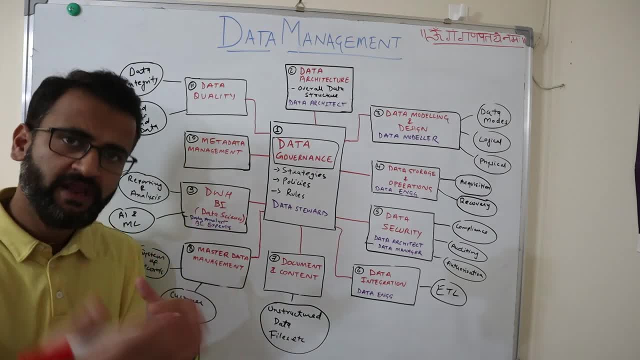 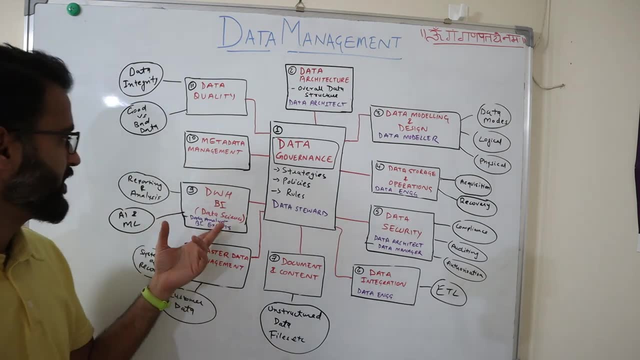 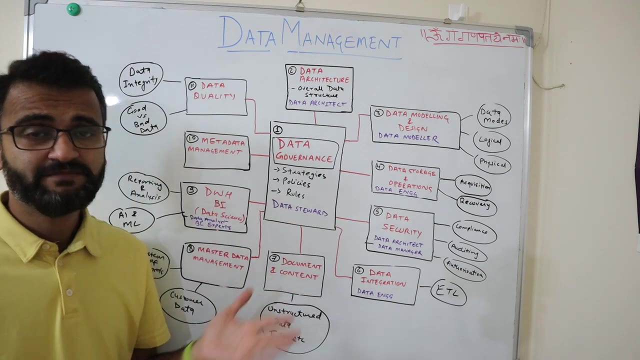 along with your data warehousing projects, you are again having a lot of artificial intelligence and machine learning projects coming in from your data science domain. Some very good roles here are data analyst, BI expert, metadata management, self-explanatory, managing all the data of the. 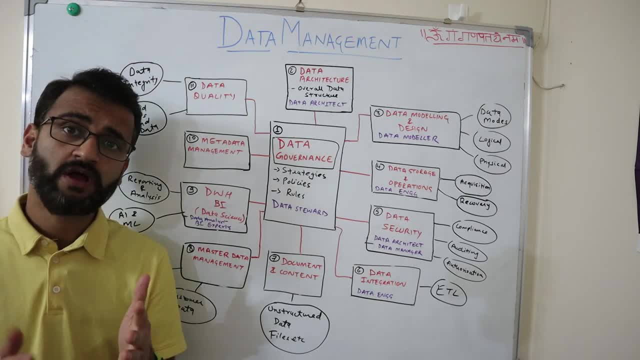 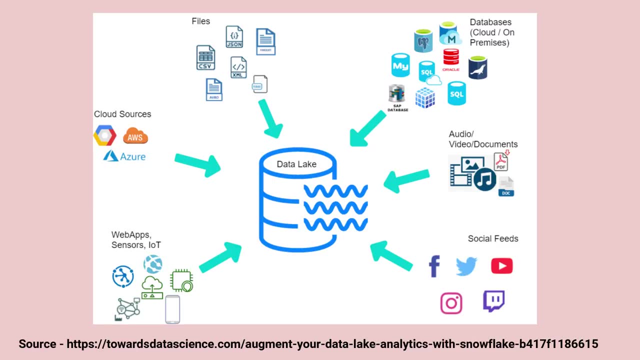 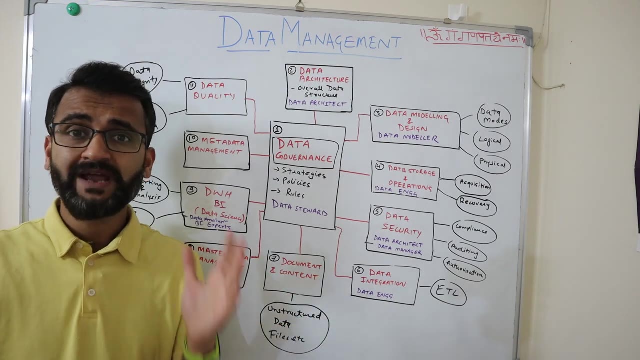 data. Take, for example, in current scenarios now, when you have data lake environments coming up okay and you are pouring all your enterprise data in your data lake from desperate systems, so it is very much possible that your data lake could become a data swamp because you might have 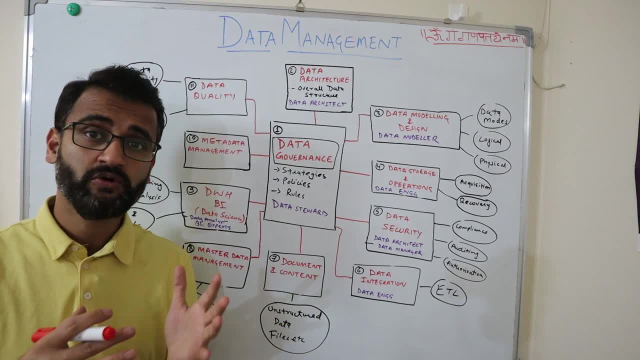 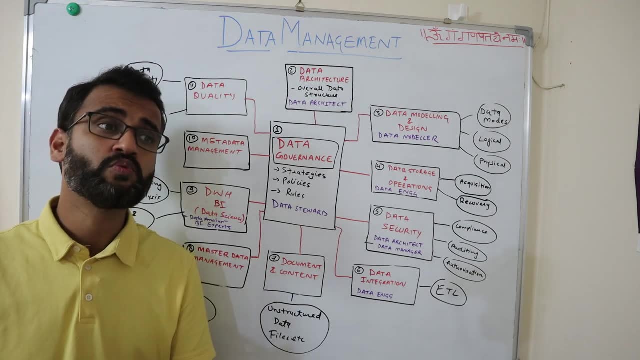 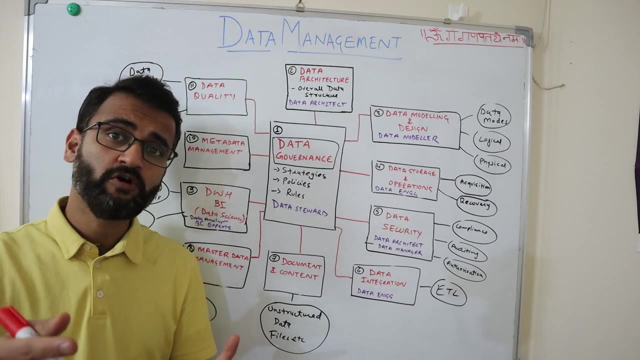 data redundancy and you might have garbage data poured into your data lake. Because why? because there is no metadata management. there is no clear answer to as to why this data has come in at first place and why it is lying here, whether we have a very exact, very copy of this. 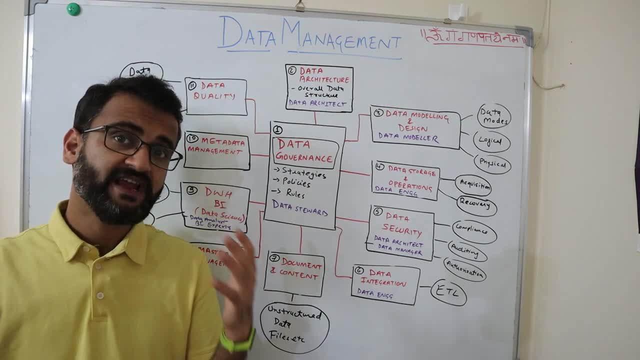 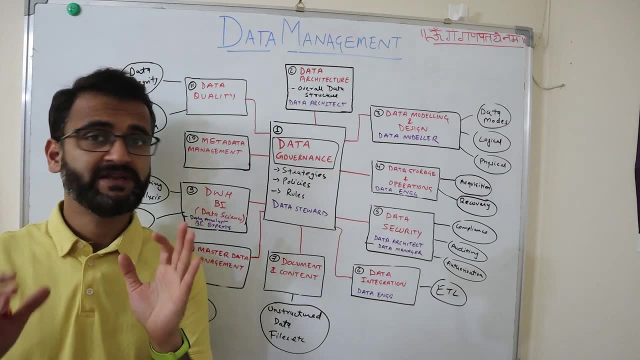 data lying somewhere else. So those kind of things can be, you know, managed with metadata management. it's very important, sometimes overlooked because people tend to focus on important aspects of getting the data to the customer, but that's not the case. So I think it's very important to have 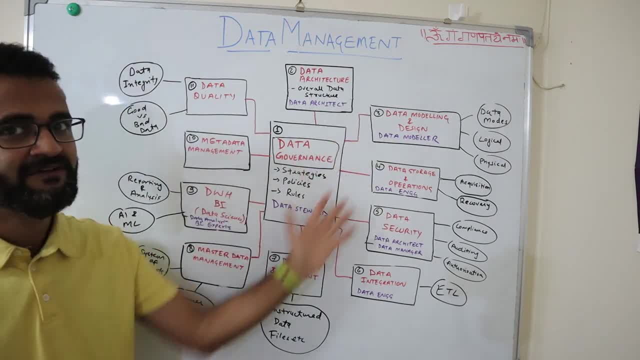 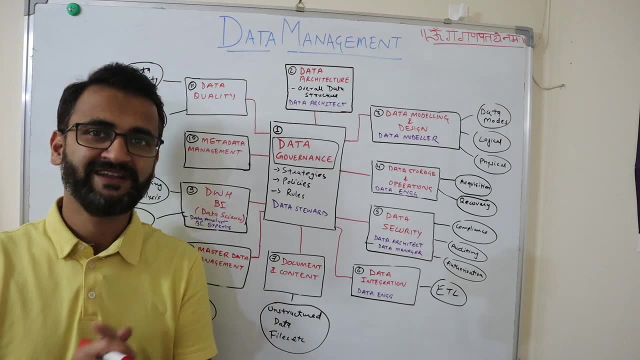 data governance in your data lake. So that's where data governance comes into picture. as you can see, it is connected with every area, so data governance is the area which will ensure that you are not taking this for granted or lightly. So it's a very important area, guys. metadata management and last, 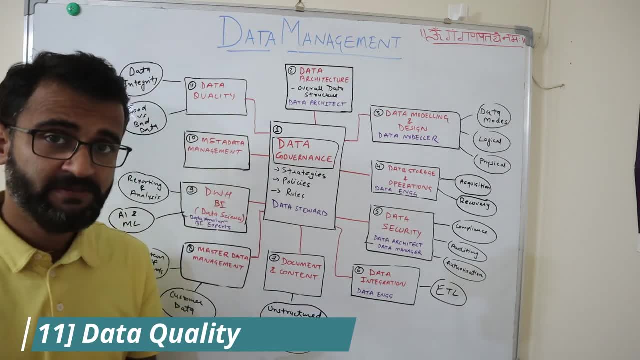 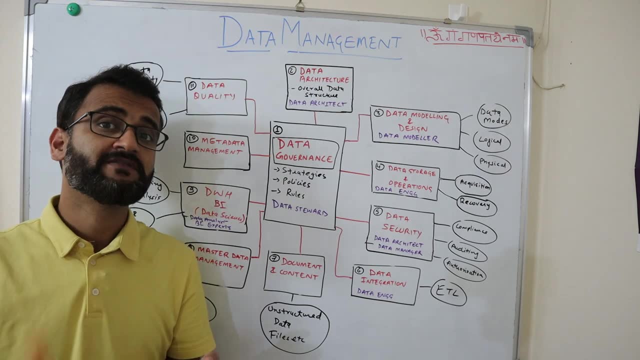 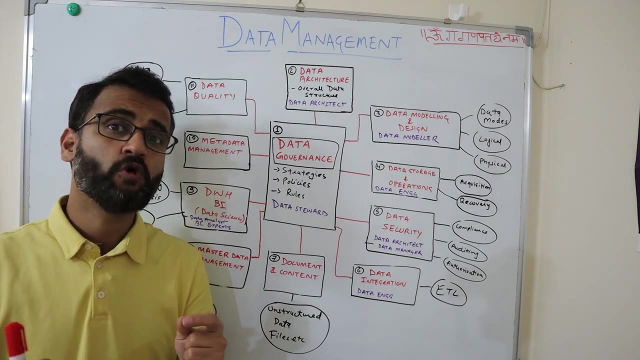 but definitely not the least, is data quality. Name is again very simple and straightforward. it manages and ensures that you know how to define good data versus bad data, how you ensure that data integrity is in place. So whenever your data quality is compromised, then there is no matter how good data pipelines you have. 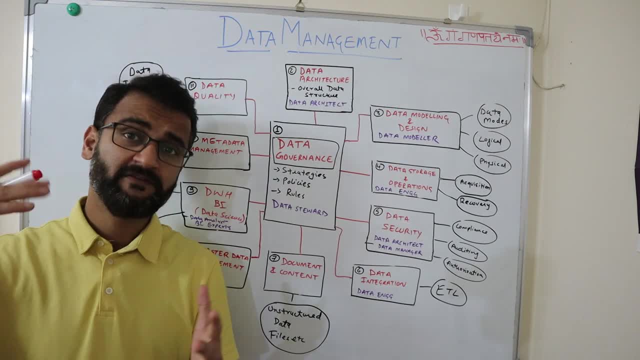 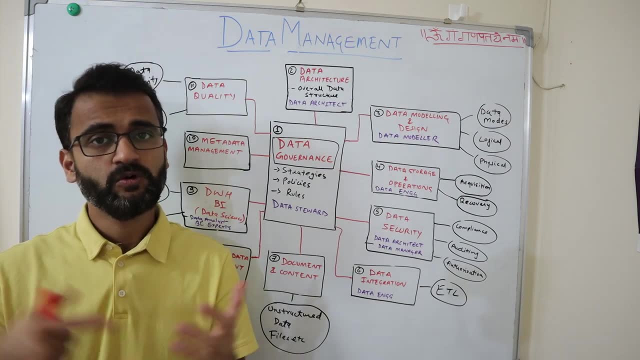 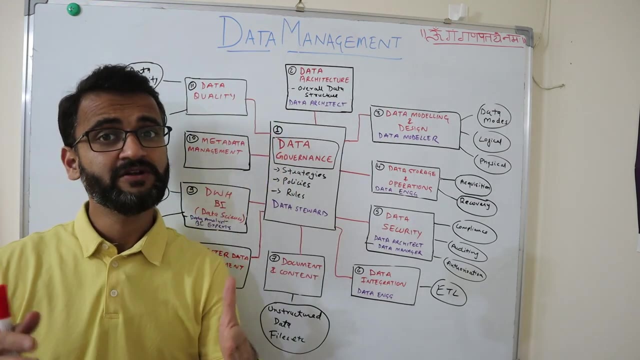 no matter how good data frameworks you develop, if your data quality is not good, then you are not returning the actual value to the business. So data quality is something which I think is maintained at every level, but then again, if there is a separate area, looking into it and again with the 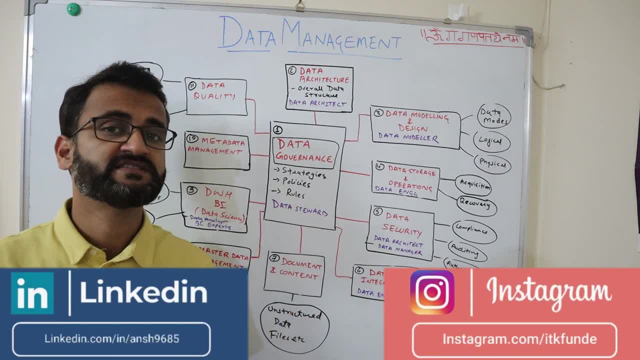 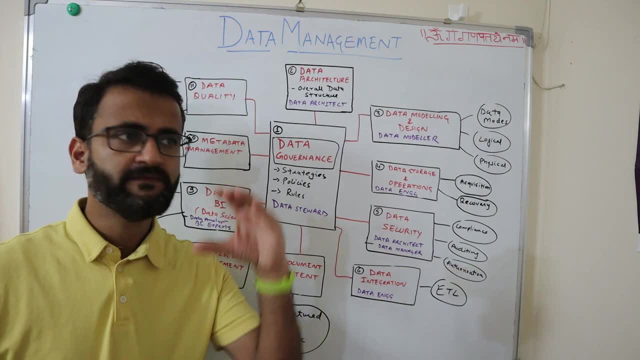 under the governance, data governance model, then definitely there is a lot of data that needs to be taken care of and that's why we say that in the cloud we have seen that people tend to tag the data with a standard. so, based on the data quality, the data freshness and data you know, correctness, you can